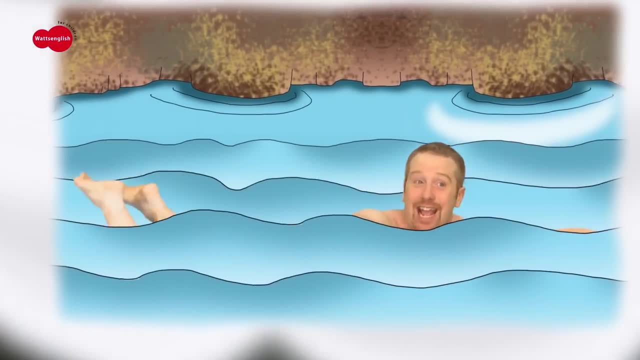 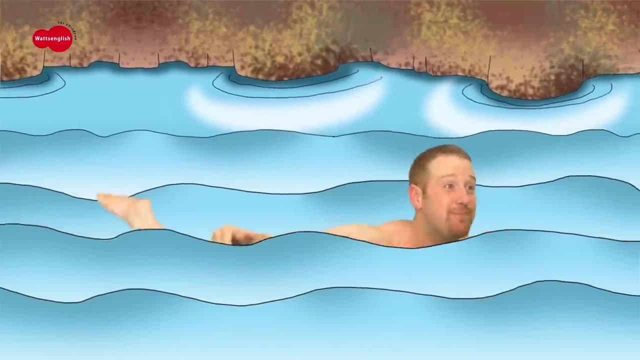 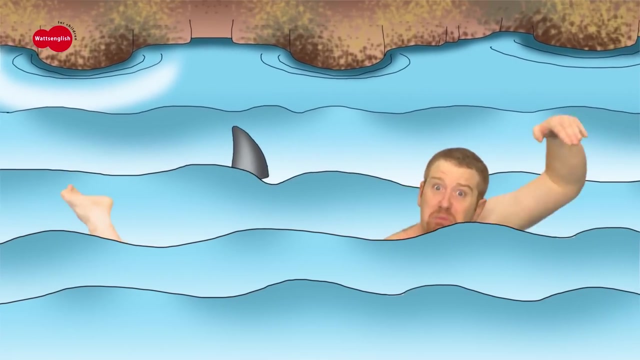 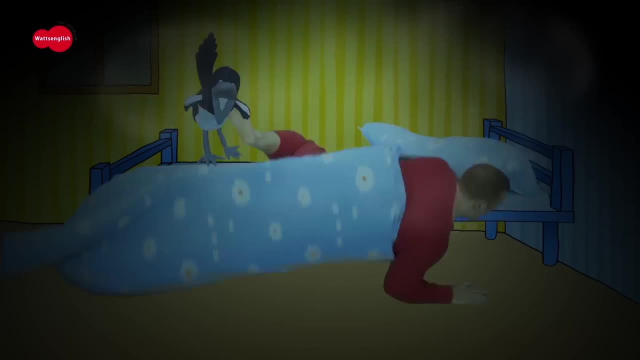 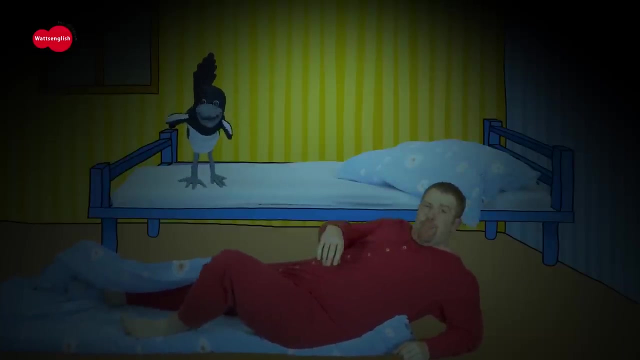 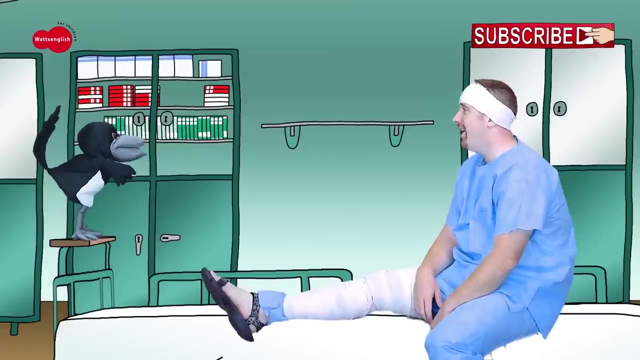 Swim Swim, Swim, Swim, Swim, Swim. Hey, hey, It´s time to say bye, bye, Hihi. Oh, by the way, Yeah, OK, Uh, It´s Steve and Maggie. Hello Steve, Hello Maggie. Oh, hello boys. 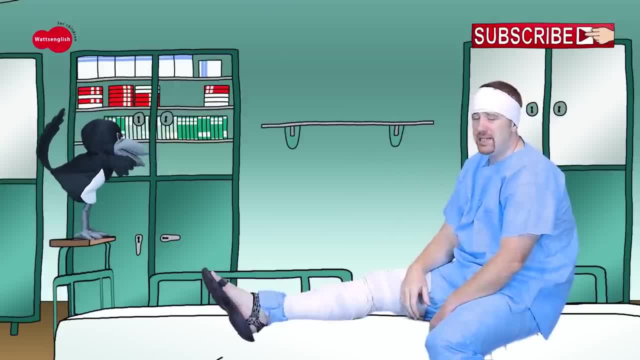 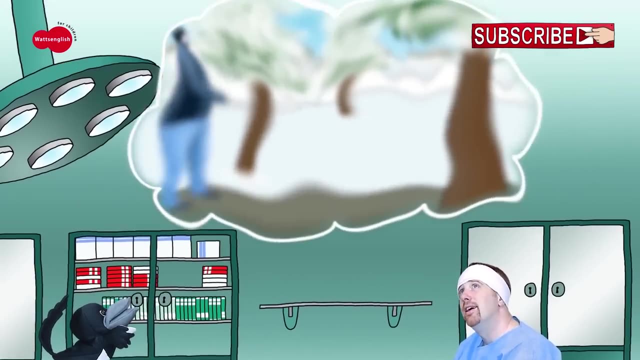 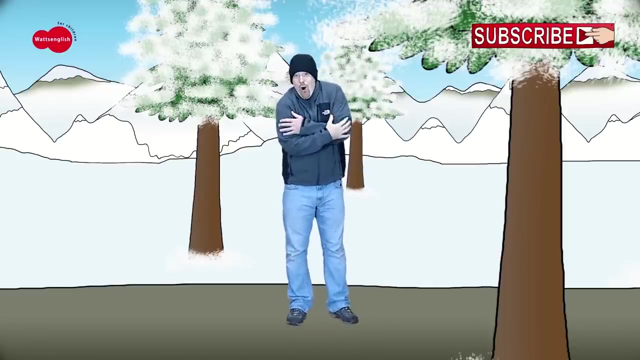 and girls, Hello, Hi, I´m not happy today. Oh dear. No, What happened, Steve? Well, I went on holiday in the mountains. First I wanted to go for a walk, but it wasn't fun. Walk, walk, walk, walk. Hey hello, Haha, Look, it's cold, but it's sunny- A good. 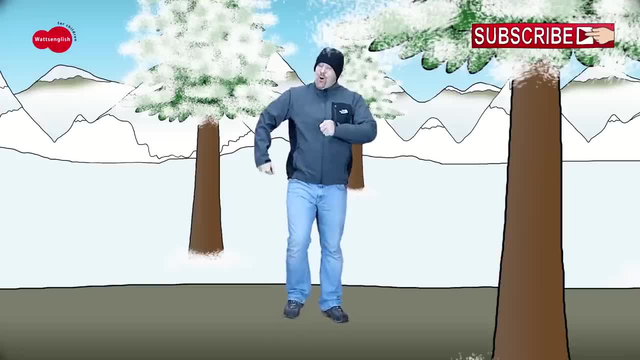 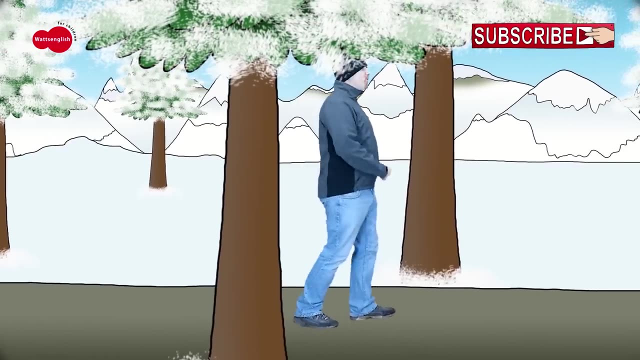 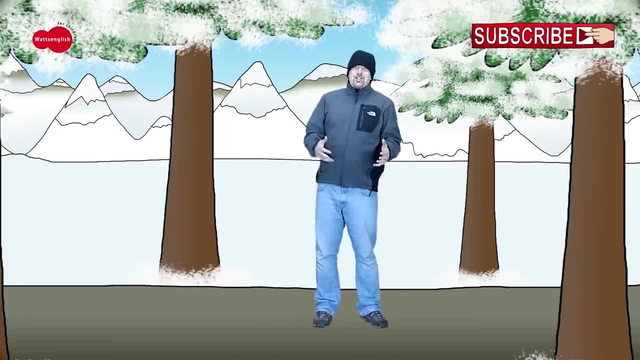 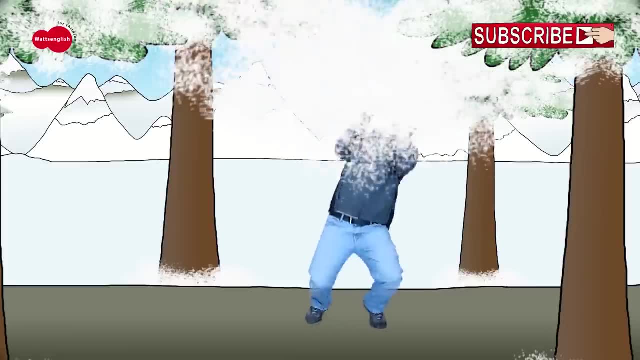 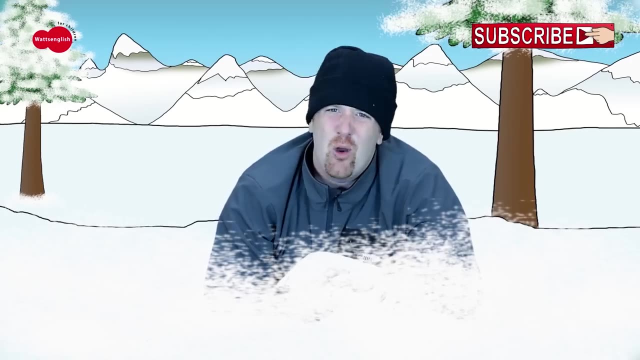 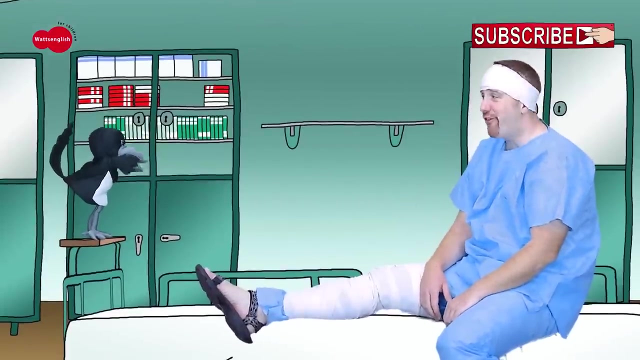 Hey, Wow, Look at all this snow. Hey, Hey, listen, What's that? Oh, I don't want to walk anymore. Haha, That's funny. Okay, Maybe that was funny under the snow. Yeah, Haha, But then. 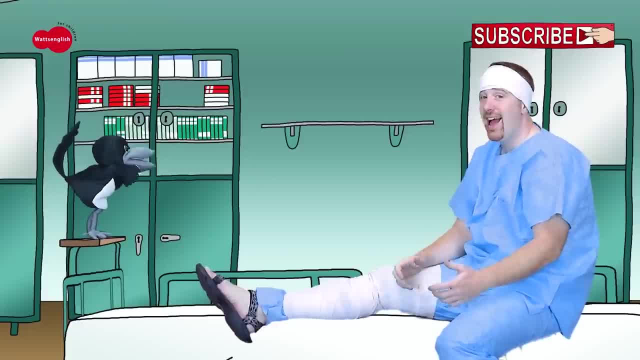 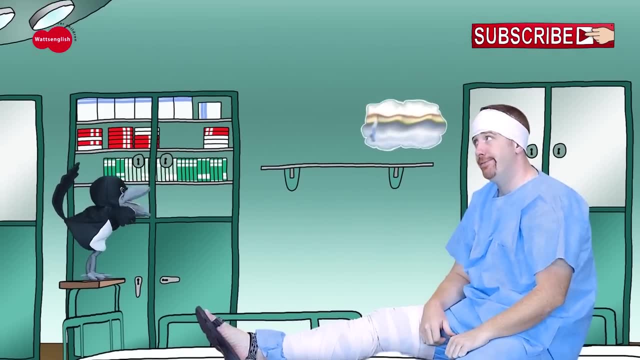 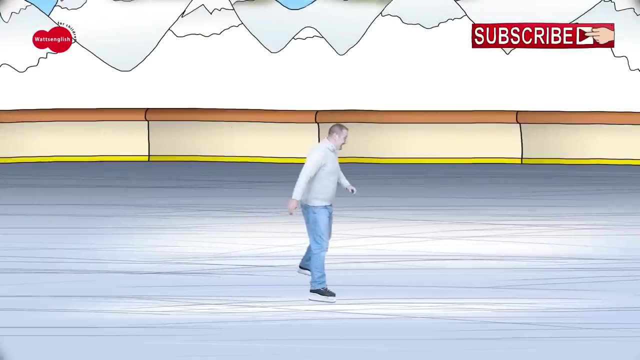 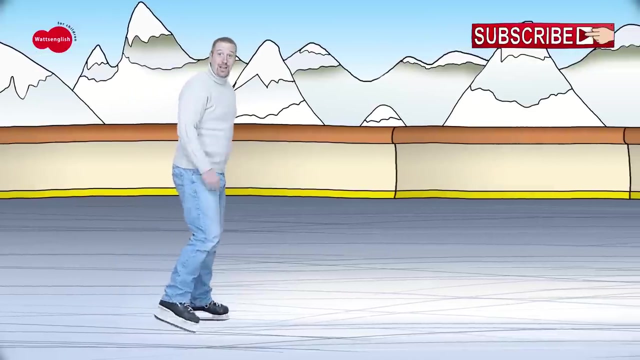 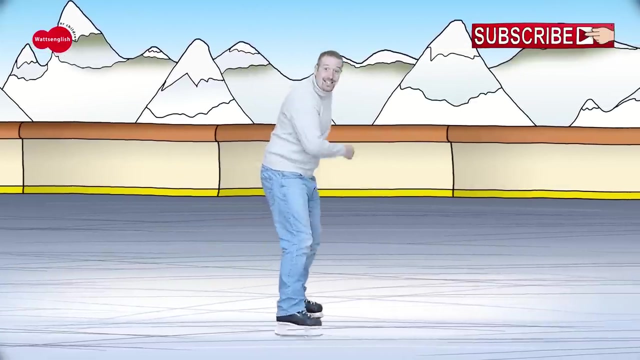 it got worse. Oh, what happened? Well, I wanted to skate, But that was a bad idea. Haha, Hey, look, Hahaha, Skating. Hey, Skate, skate, skate, skate, Skate. Yeah, Can you skate with me? Stand up, Come on and skate, Skate, Skate, Skate, Skate, Skate. 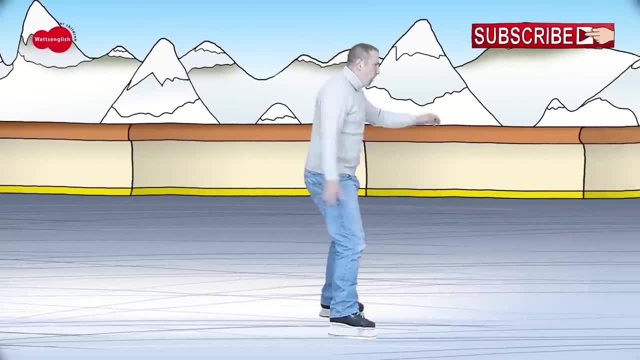 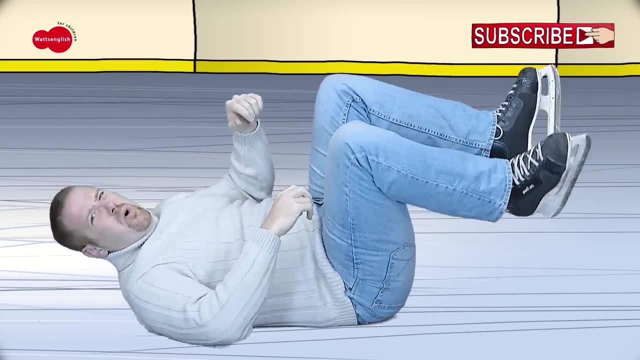 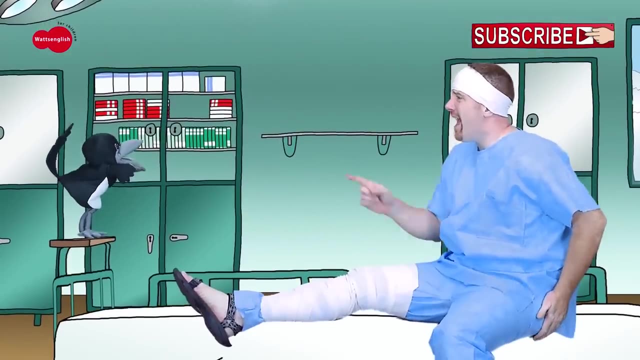 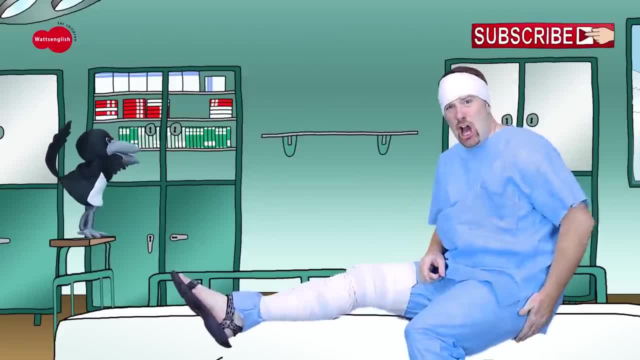 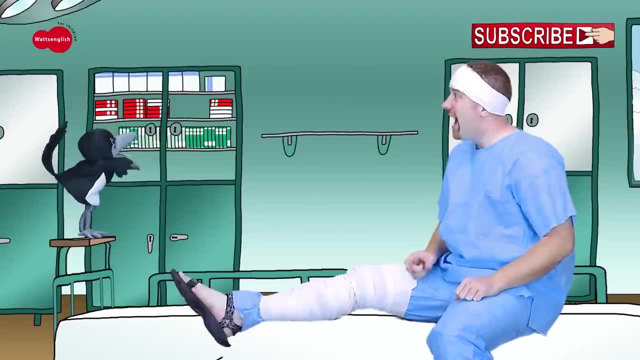 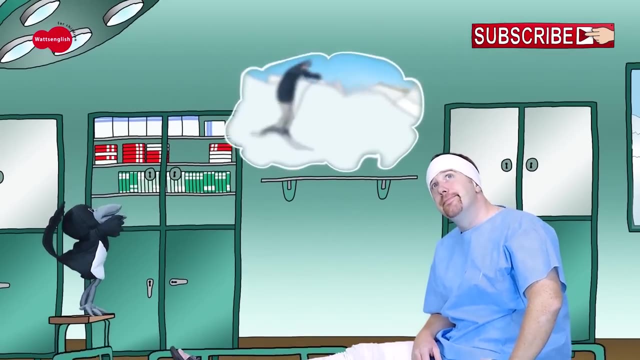 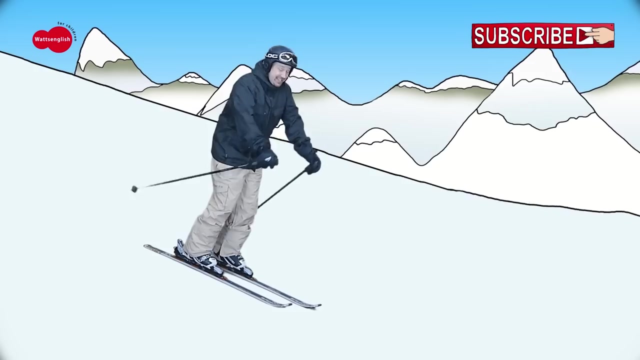 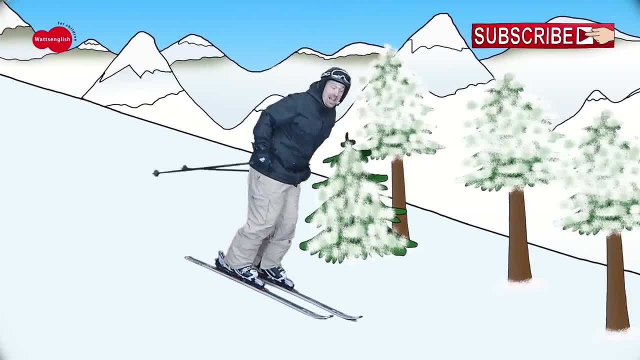 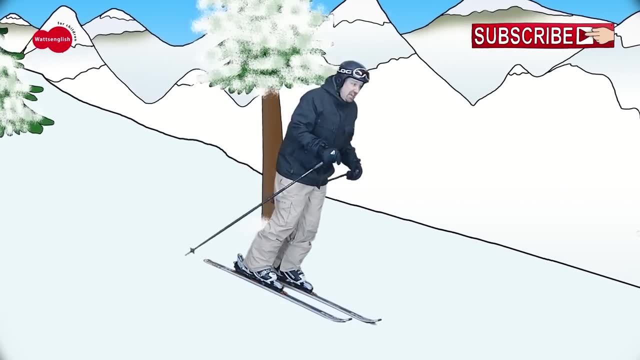 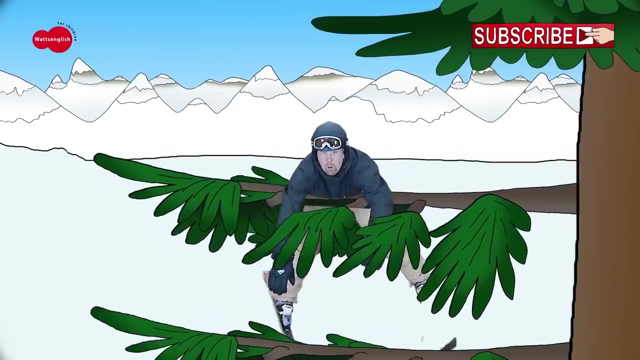 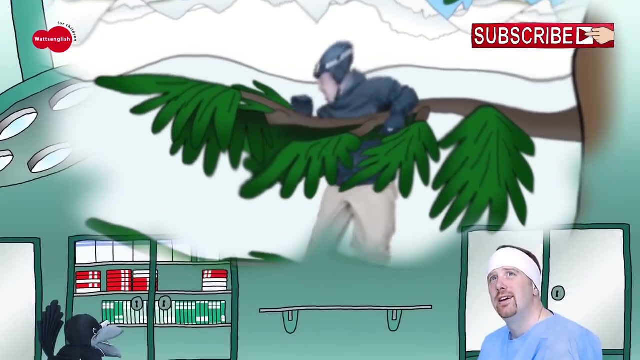 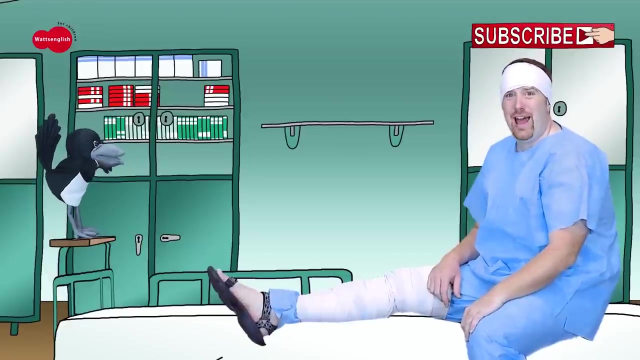 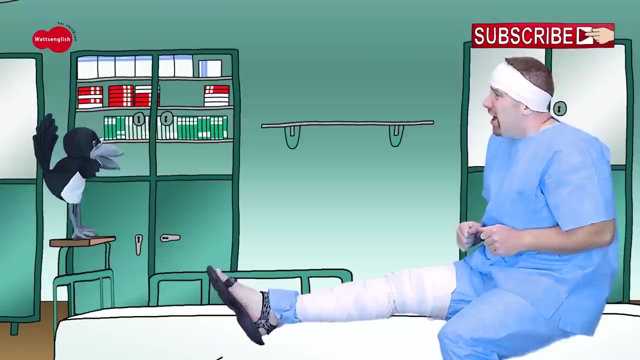 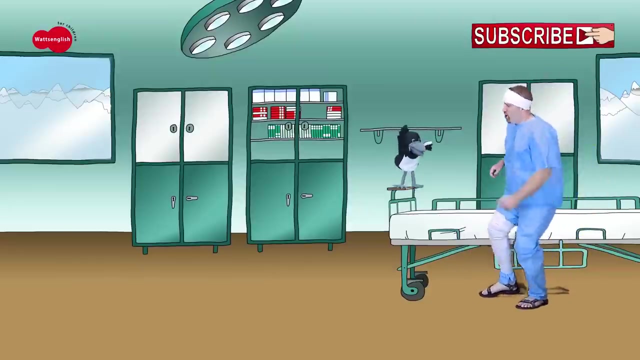 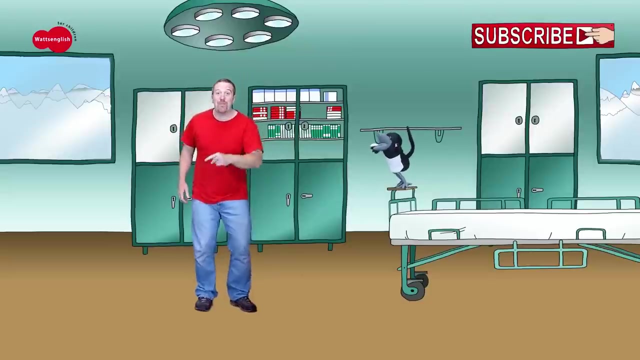 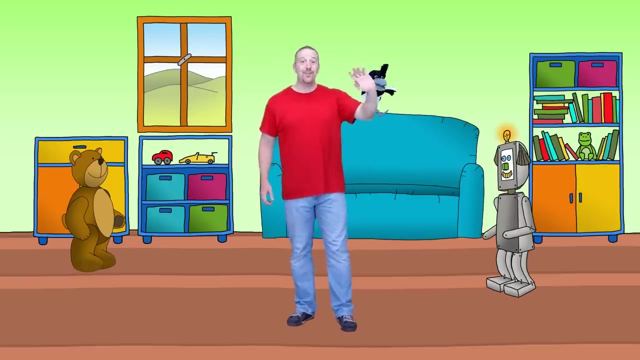 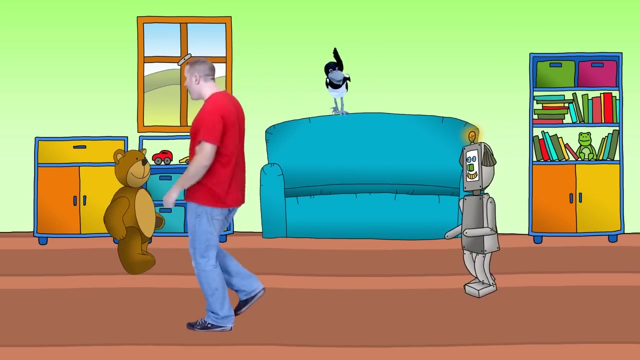 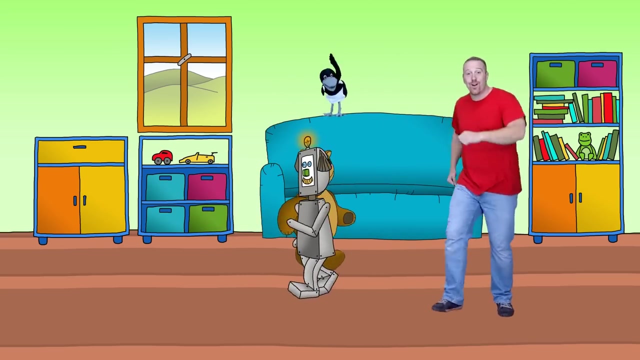 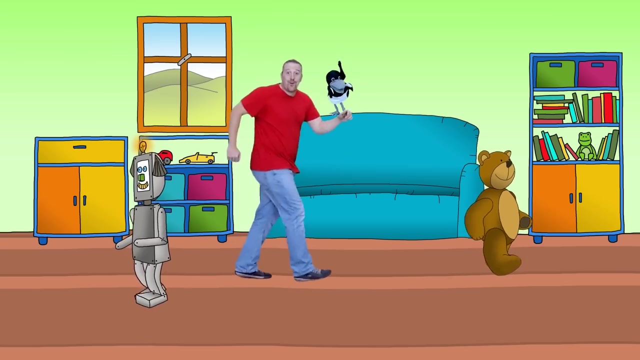 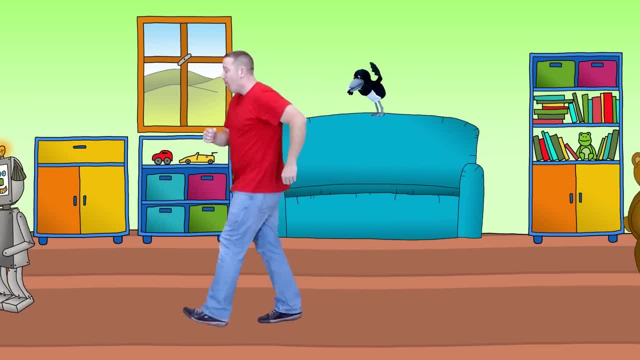 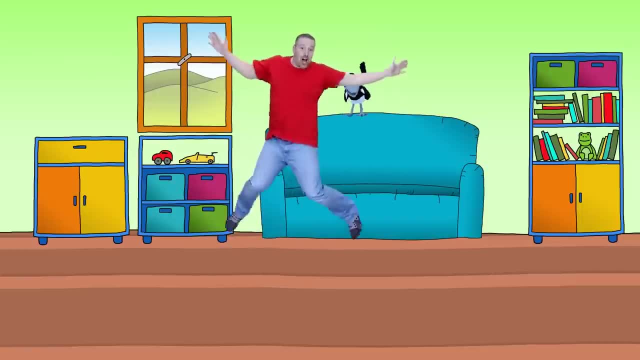 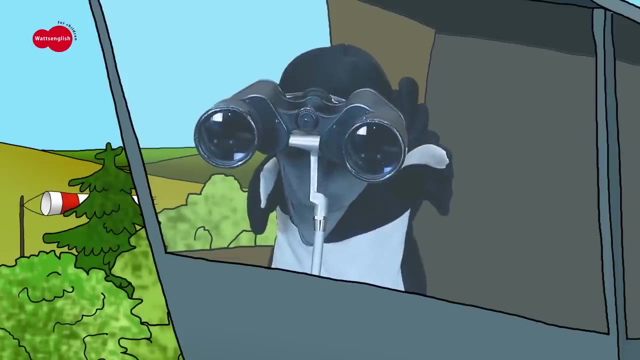 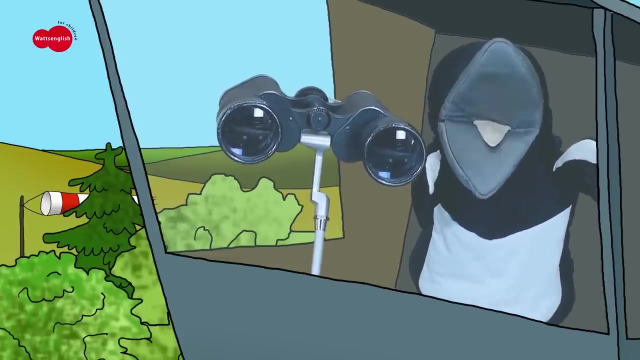 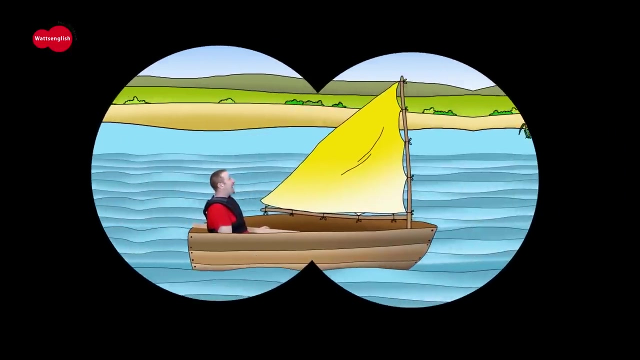 Let's walk, walk, walk, walk. but be careful now and stop. Come on, let's jump, jump, jump, jump. it's Steve and Maggie. Oh, hello, boys and girls. hi, where is Steve? Wow? 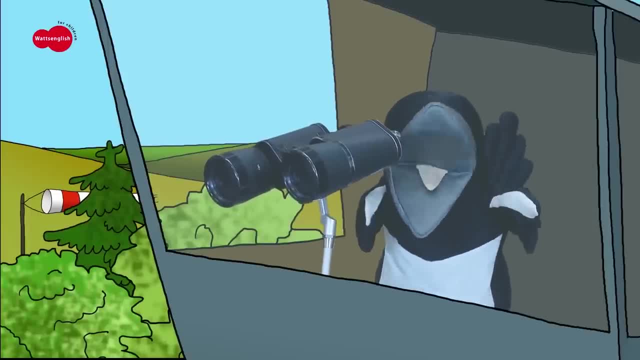 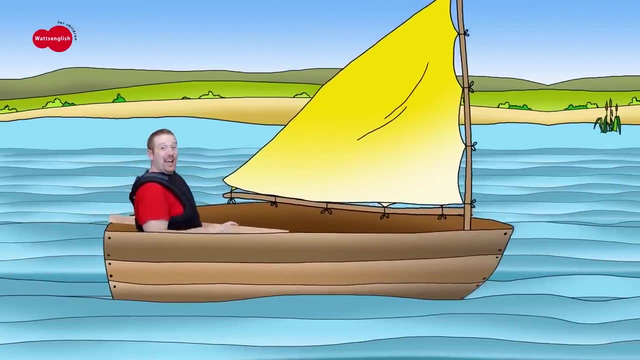 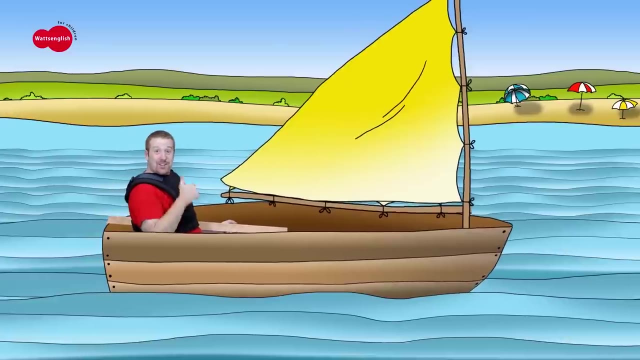 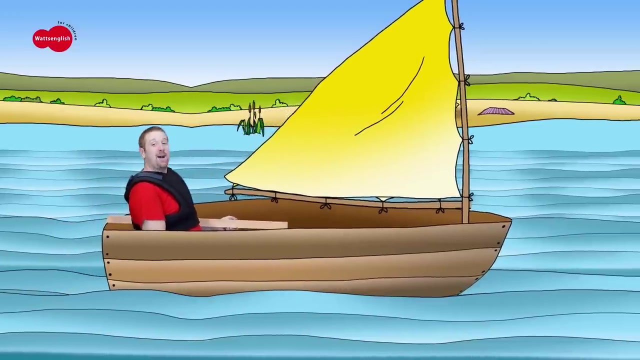 Oh, look, he is on a boat. ha-ha, yeah, Wow. Oh, hello again. look, I am on a boat, Yeah, it's great. ha-ha, Say with me, it's a boat, Come on, it's a boat and again it's a boat, yeah. 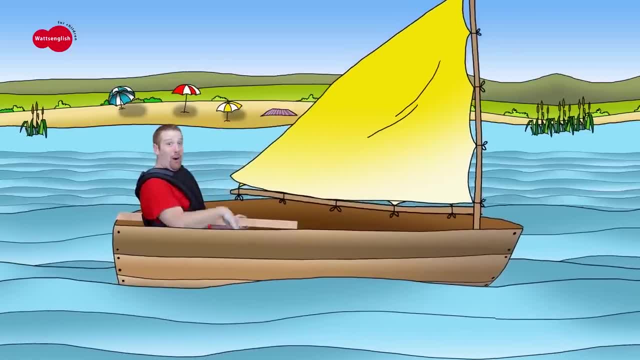 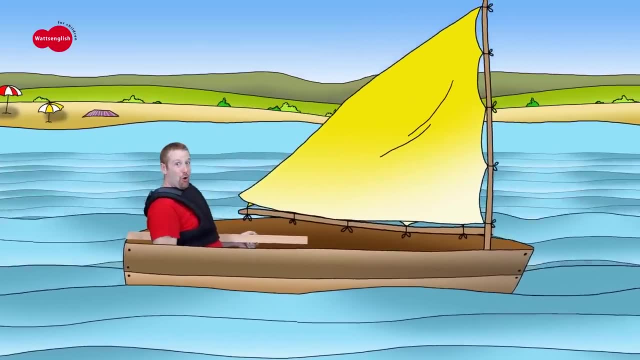 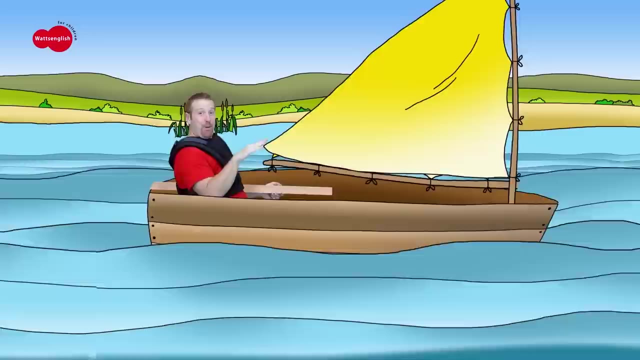 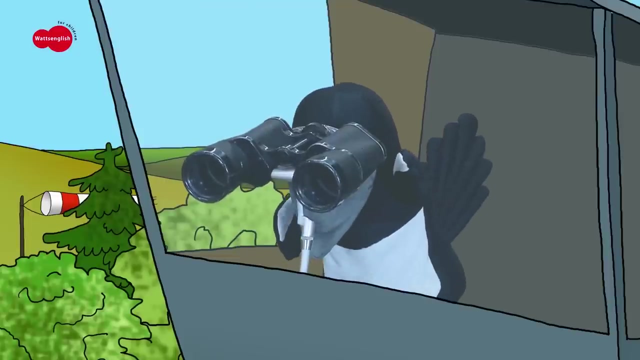 Oh, the waves are getting bigger, oh-oh-oh, Say with me up here, say it's a boat, oh-oh-oh, down here it's a boat, ha-ha-hey. Oh, back up here it's a boat, and again down here, oh, it's a boat, yeah, ha-ha-hey. 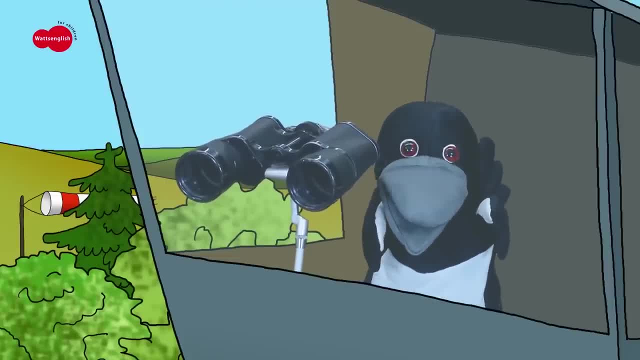 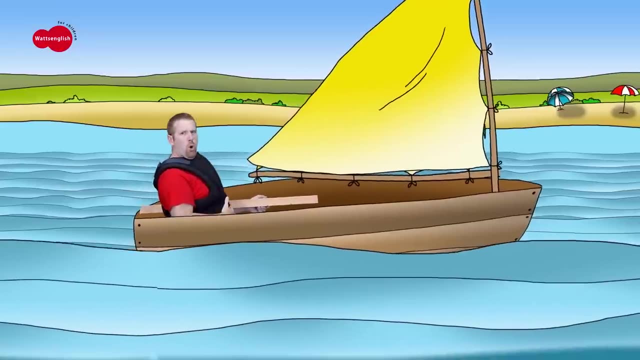 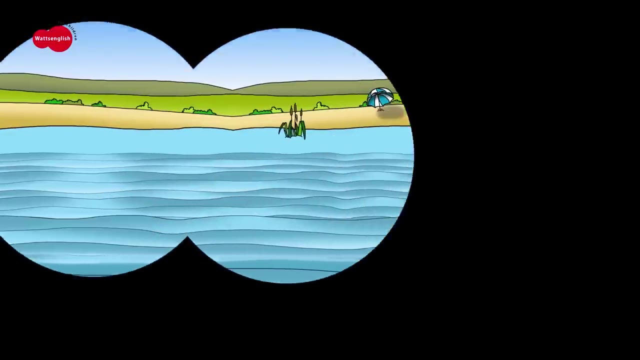 it's a boat. ha-ha it's a boat. yeah, yeah, Well done. Oh, oh dear. oh, I don't feel so good. oh, ha-ha, wow, what's that? Hey, Oh, no. 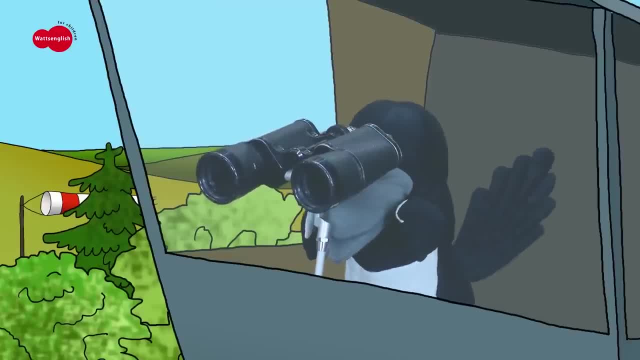 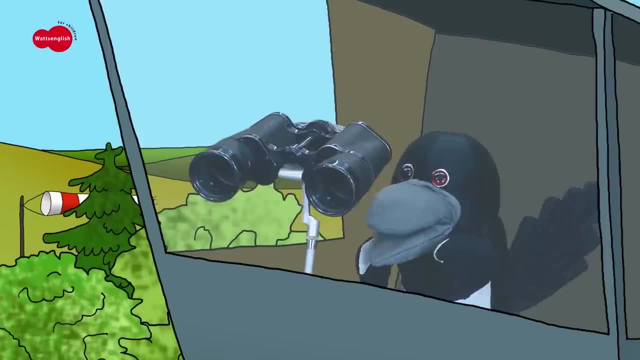 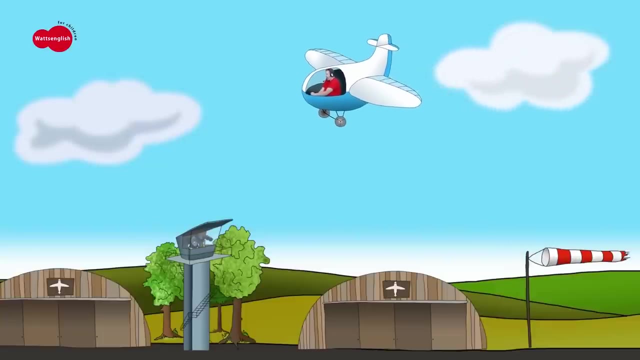 Oh, Oh, oh. where's Steve now? Hmm, Where's Steve? Where is he? I don't know. Hmm, Ha-ha-ha-ha, Look up, Ha-ha, Steve's up in the sky, Hey. 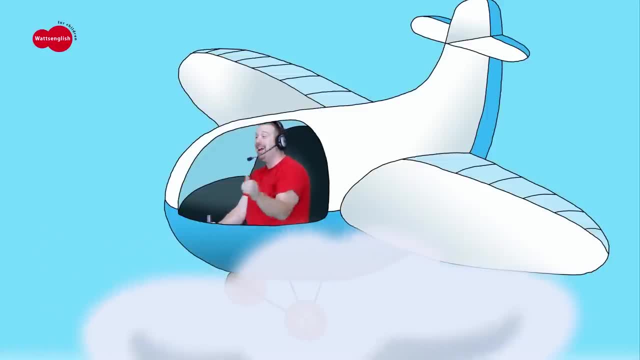 Ha-ha, Ha-ha-ha, Hello, Look, Ha-ha, Ha-ha. What is this? What is it? Yeah, it's a plane. Whoa, It's a plane, Haha, Haha. So say with me: Come on, It´s a plane, It´s a plane Again, It´s a plane, Yeah. 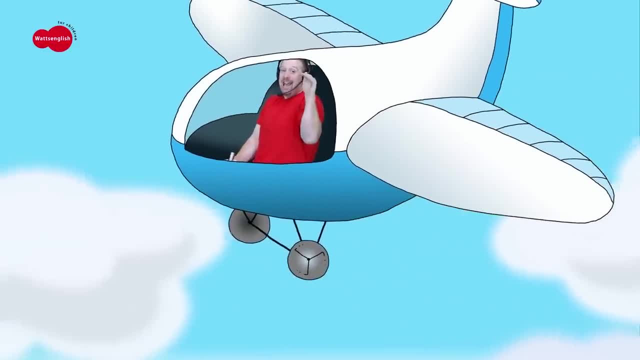 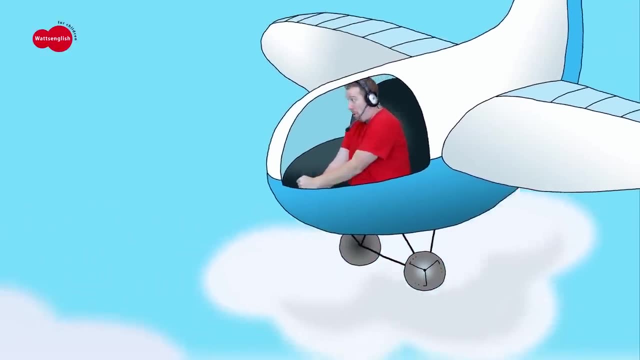 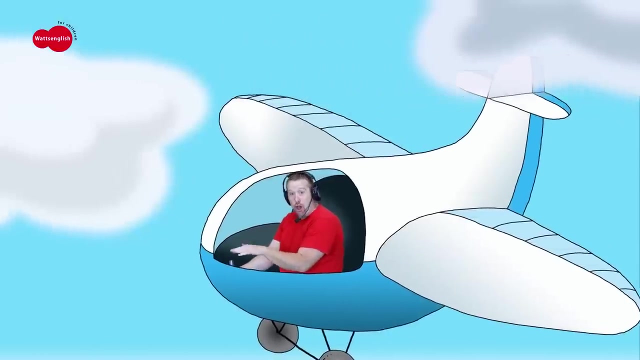 Watch this: Go up, Whoa, And we say It´s a plane, It´s a plane, Again It´s a plane. And down And say It´s a plane, It´s a plane, It´s a plane, Yeah, Look, Watch. 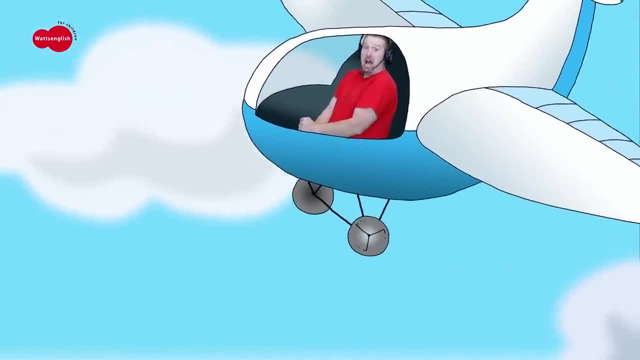 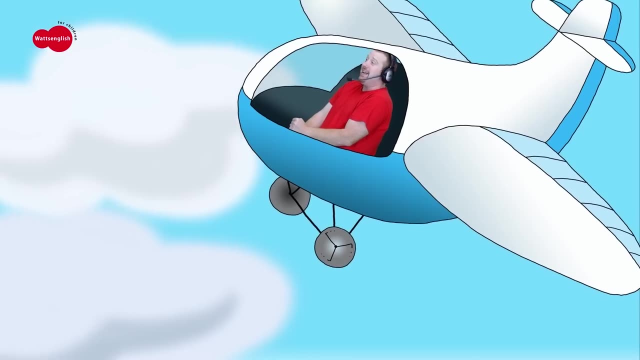 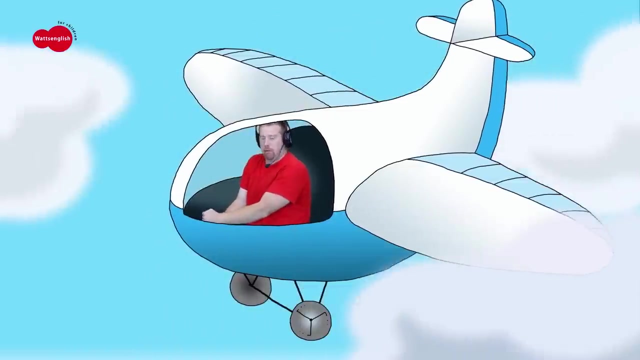 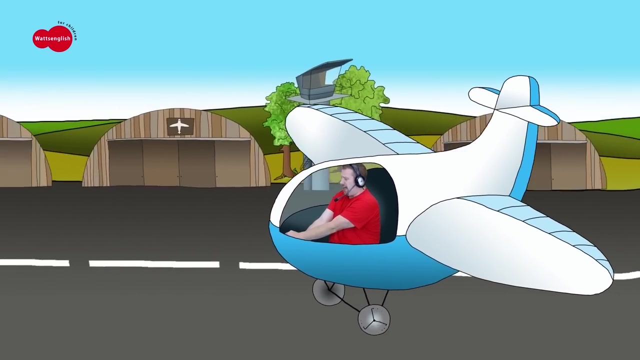 Up, Ha-ha, It´s a plane, And down, It´s a plane, And up It´s a plane. Yeah, And down, Oh, It´s a plane, Oh, Oh, Oh, I don't feel so good. Oh, Down, down, down, down and stop, Oh dear. 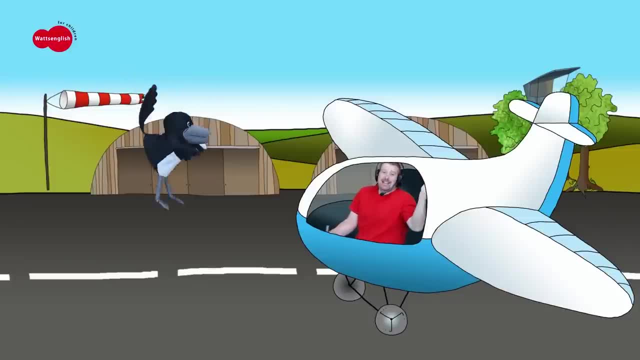 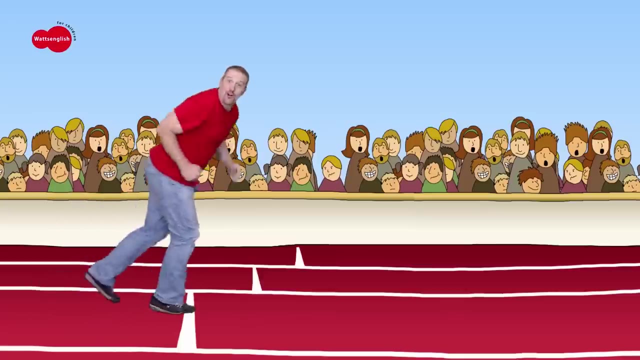 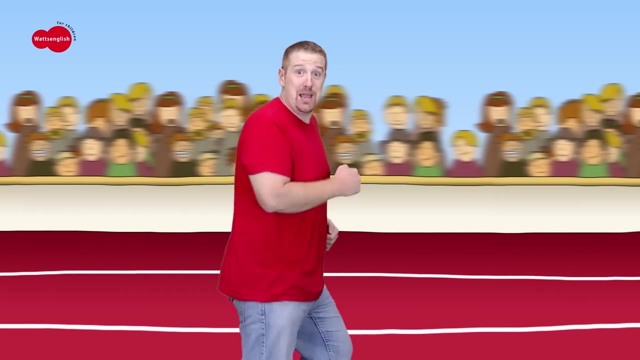 Bye, bye, See you next time. Bye bye, Up down, up, down, up down. No problem, Yes, Maggie, Well done, It's Steve and Maggie. Hello, Come on, Let's run, Run, run, run, run, run with me, Run, run, run, run, run with me, Run, run, run run. 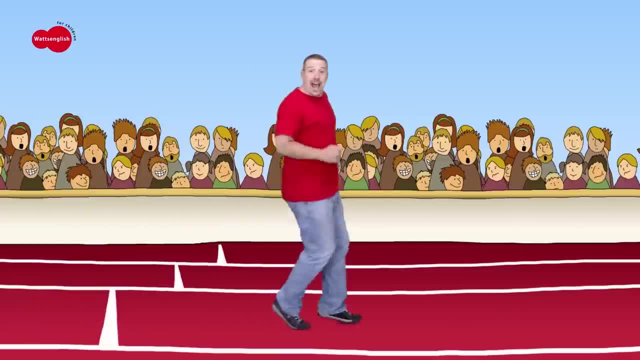 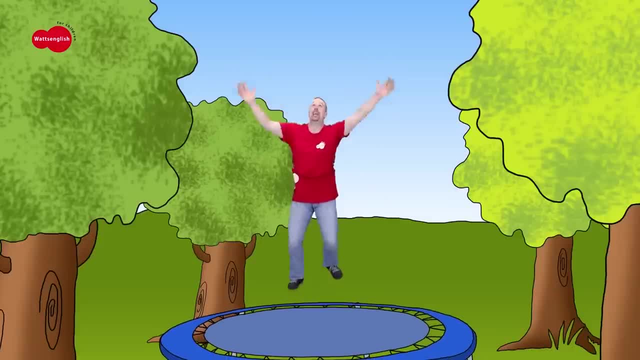